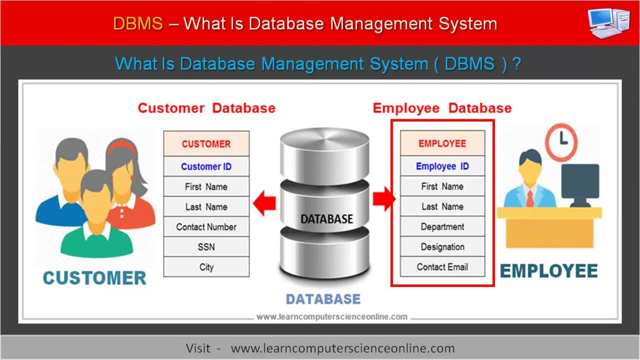 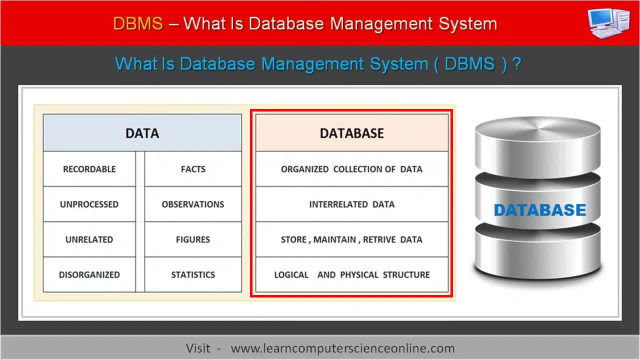 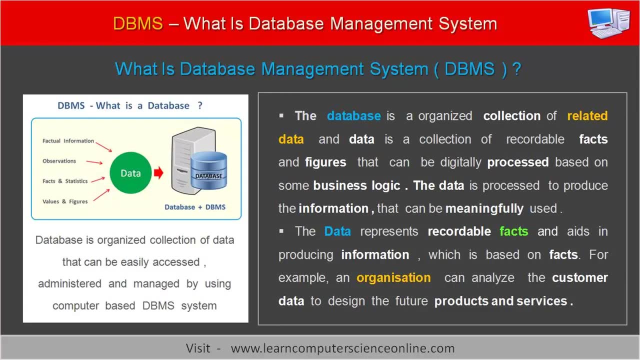 might include name, data of birth, address, designation, salary and so on. Let us now discuss the meaning of term database. The database, in simple terms, is the organized collection of interrelated data that can be efficiently stored. 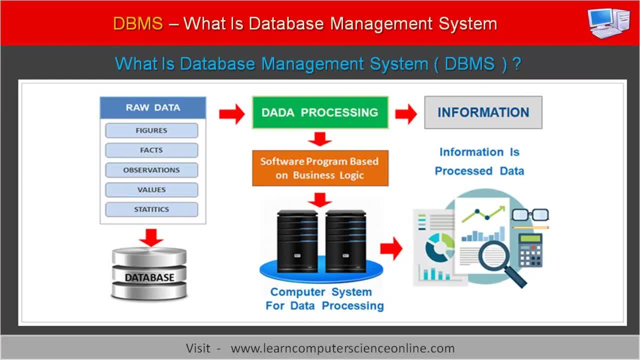 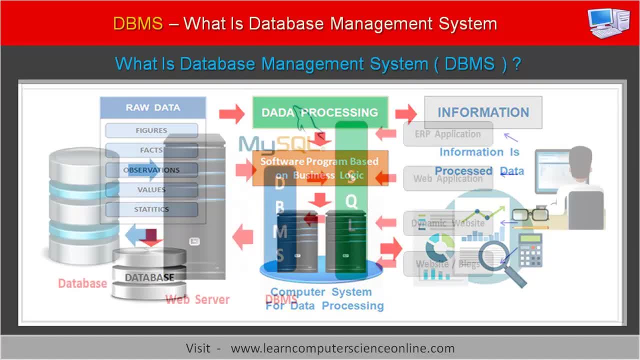 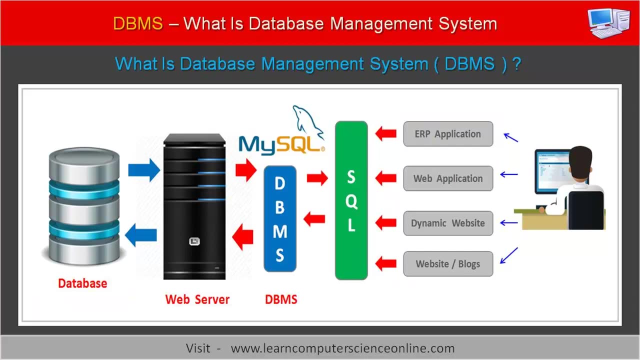 accessed and manipulated. The database offers many advantages and the most efficient way of storing and organizing the data. The database is an important element of most software applications designed to store, access and process the data with the help of. 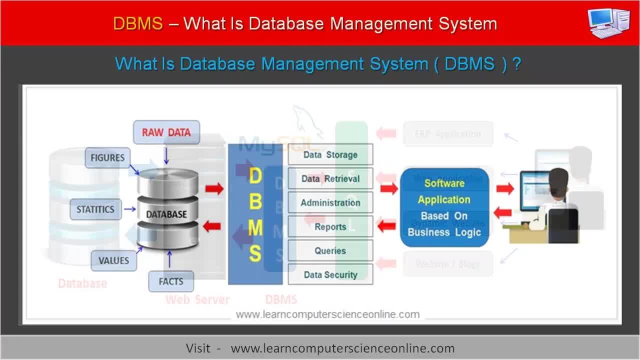 any DBMS software application. Let us now discuss what is a database management system. The term DBMS stands for database management system, which is a software designed to perform various database operations. The database operations performed by the DBMS includes: 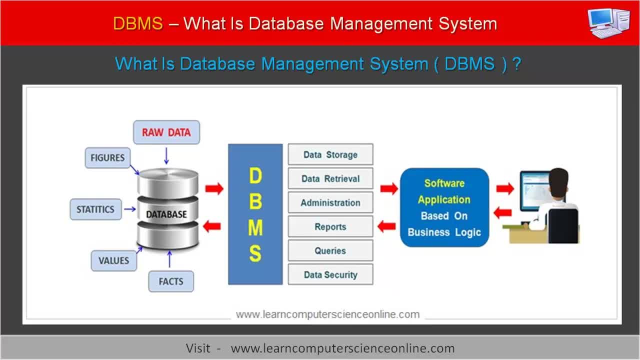 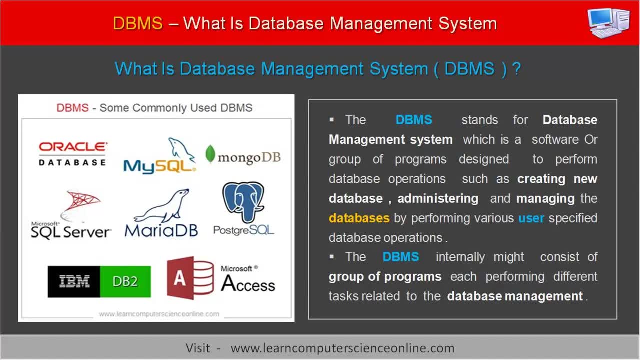 creating new databases, administering, managing and manipulating the databases. The database manipulation operations includes creating new database, modifying the tables, adding and deleting the data in the table and other such user specified database operations. The DBMS internally might consist of: 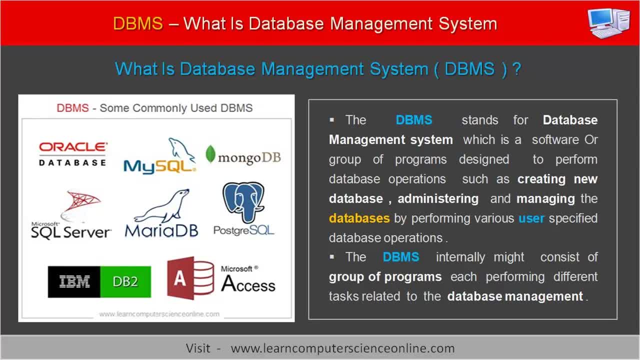 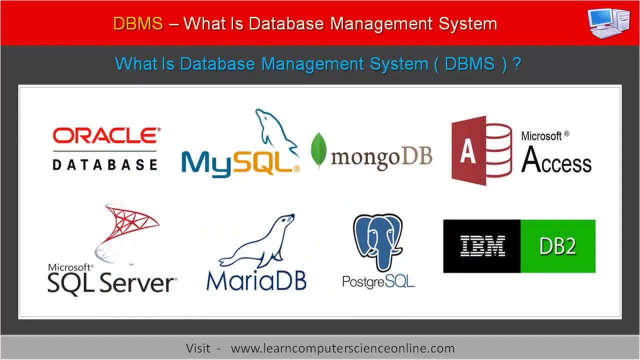 group of programs. Each of these program performs a different task related to the database management. Some of the most commonly used DBMS includes MySQL, extensively used for web applications, Oracle, Microsoft SQL Server, IBM DB2,, Microsoft Access, MariaDB. 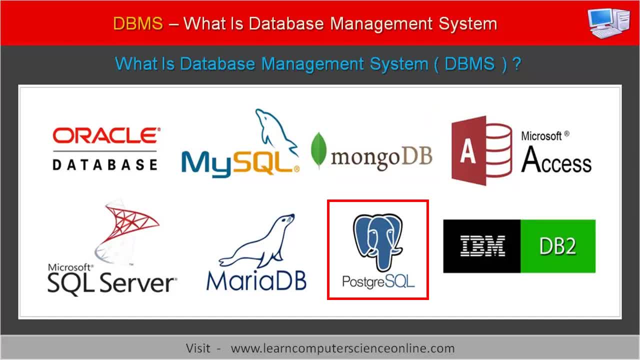 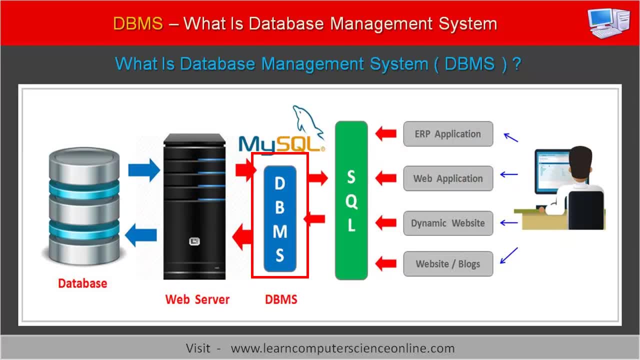 MangoDB, PostgreSQL, and there are many more DBMS available in the market. The DBMS also provides the necessary tools required for the design and the development of databases. The database management system is a vital component of most of the software applications. 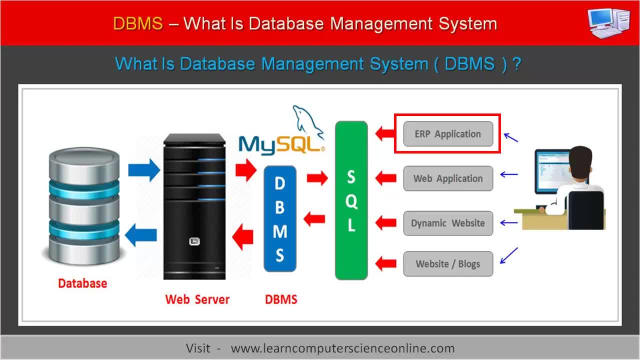 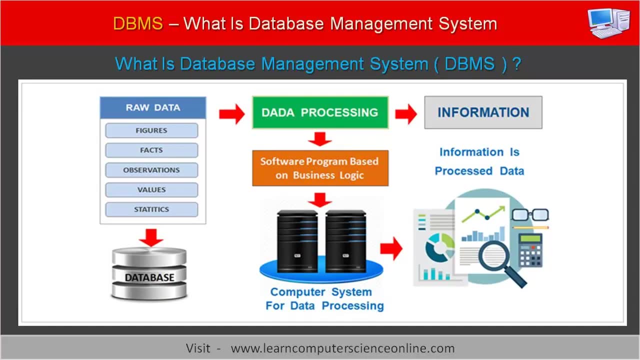 Whether you are working on a enterprise software development project or you may be developing a small website. the database design and development skills are needed in almost all software applications And therefore the DBMS knowledge is important for programmers and software developers.